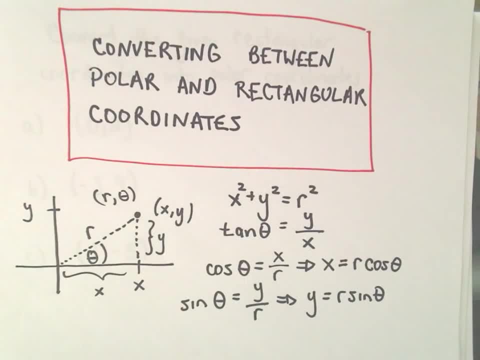 Alright. so just a couple examples here of converting between polar and rectangular coordinates. So suppose we go over x units and up y units. Well, in Cartesian coordinates our point would be x, y. In polar coordinates. suppose, well, we make an angle of theta with a positive x-axis. 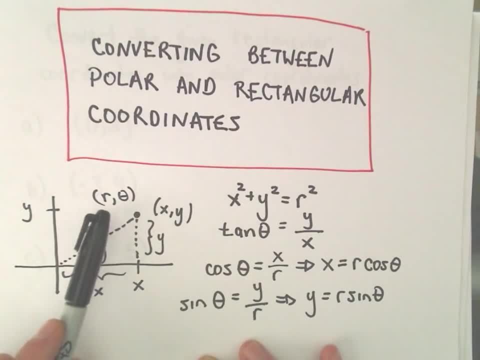 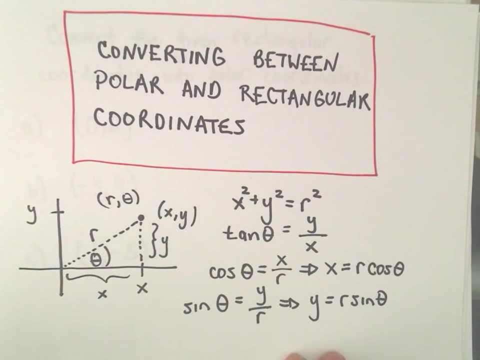 and then we go at a distance of r? Well, in polar coordinates we would label this point r theta. And again, we can just get all of these nice little relationships between polar and Cartesian coordinates just by doing a bit of geometry. 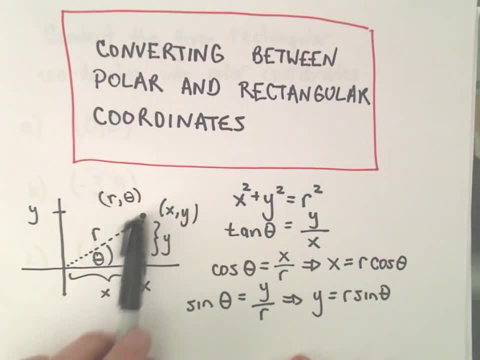 You know, you could use Pythagorean theorem: x squared plus y squared would have to equal r squared. That's our first one, Tangent's just opposite over adjacent. so tangent of theta would have to be y over x, And we can do the same thing for cosine and sine. 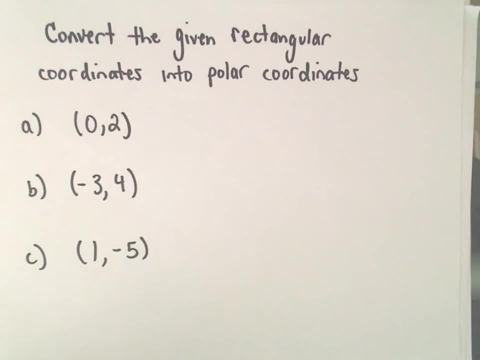 Alright, so I think I'm going to do a and b in this part And then we'll do part c in another one. So suppose we want to convert the point 0, 2.. We want to go from rectangular coordinates into polar coordinates. 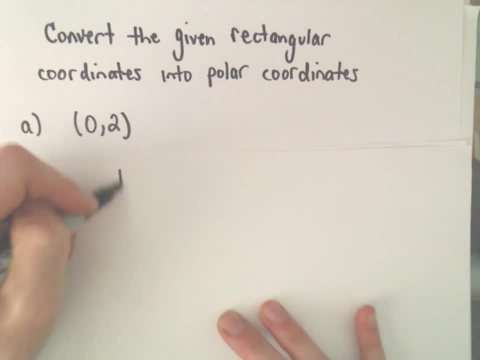 Well, we could use our formulas. I will do that on the next one. On this one, I think it's relatively straightforward. You know, if we find the point 0,, 2, well, that would be our point In Cartesian coordinates, in polar coordinates. 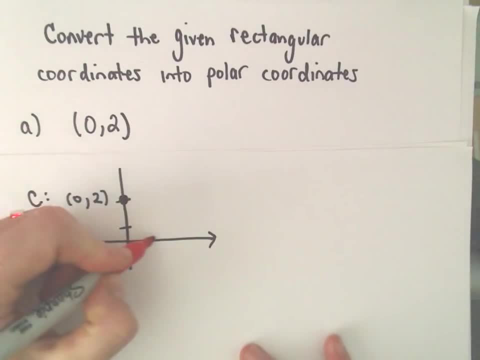 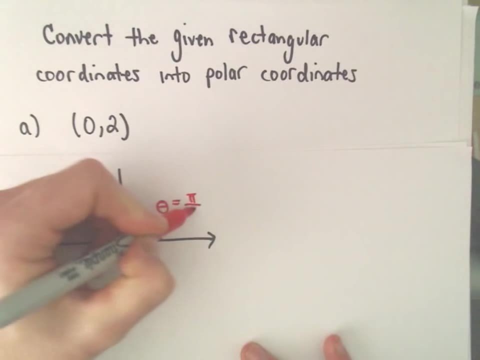 well, let's see, I guess, a couple things here. Our angle that we would make here in this case, our theta, in this case, well, theta would just equal pi over 2. And if you think about sort of that distance, you've gone out from the origin. 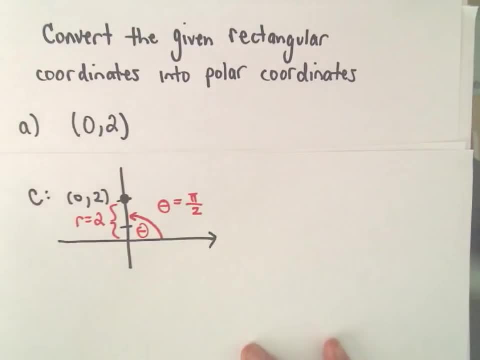 well, we're two units away, so our r value would also just equal 2.. So the polar form of that point. again we list the r value. so it says we've gone two units out from the origin, at an angle of pi over 2.. 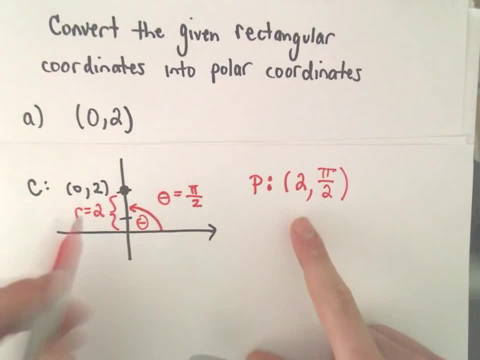 So in polar coordinates that's all we would have to do. We would say the Cartesian point represented by 0, 2.. In polar form the coordinates would be 2, pi over 2.. Or at least that would be one way of expressing that point. 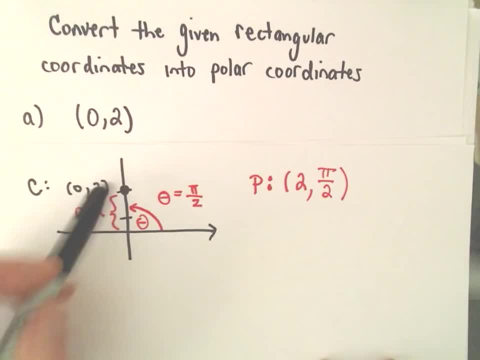 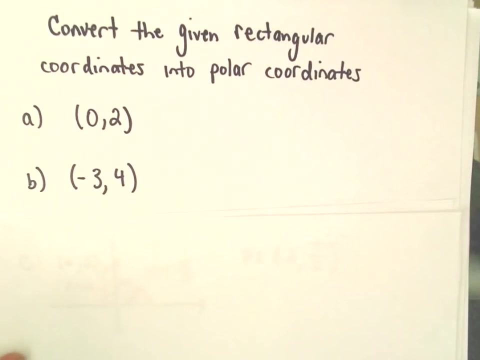 Okay, So again in polar coordinates there's infinitely many ways to represent a given point, And you know that one, to me at least, seems like the most straightforward. in this case It certainly works. Okay. So let's look at part B here, negative 3,, comma 4.. 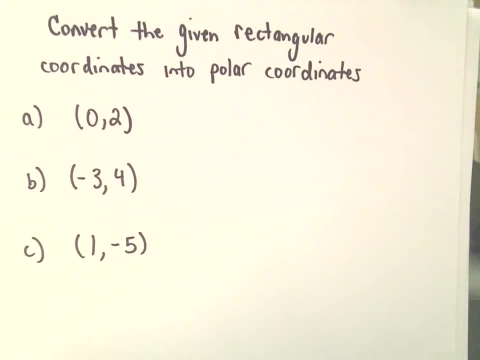 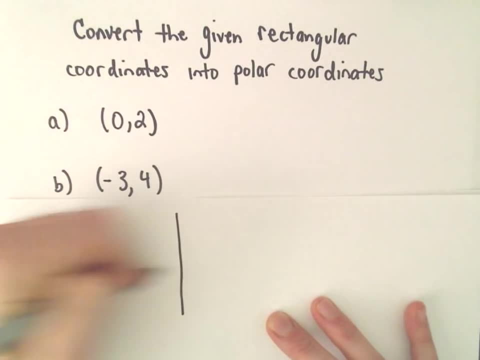 We'll do that one as well, since part A wasn't too terrible, I think. So let's see Negative 3, comma 4.. So there's negative 1, negative 2,, negative 3, and then up 1,, 2,, 3,, 4.. 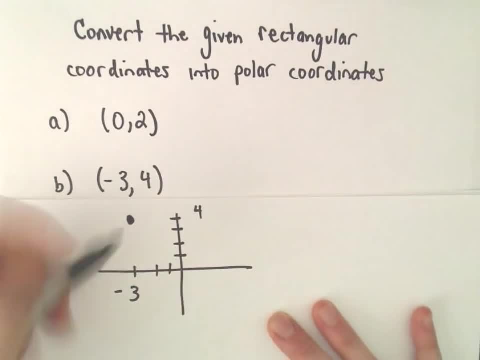 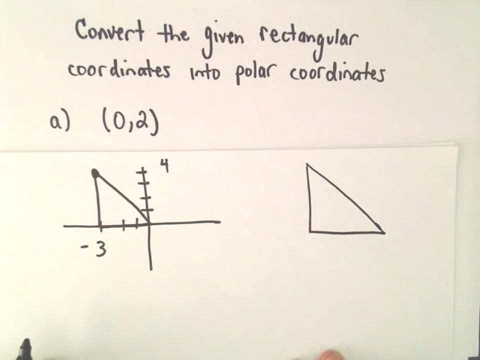 So there's our point Again, just like before. Okay, So I'm just going to make my little triangle here. I'm going to make my little triangle And I'm going to do a couple things. I'm going to call this my angle alpha. 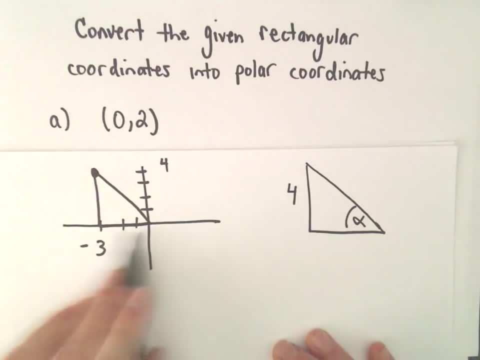 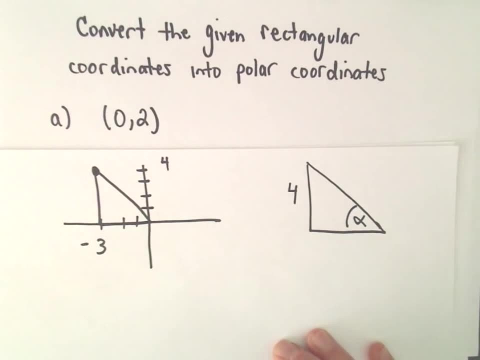 And okay. so again, we went up 4 units. I know that this is a negative. you know, we went negative 3 units to the left. Well, I guess we went 3 units to the left, which gives us negative 3.. 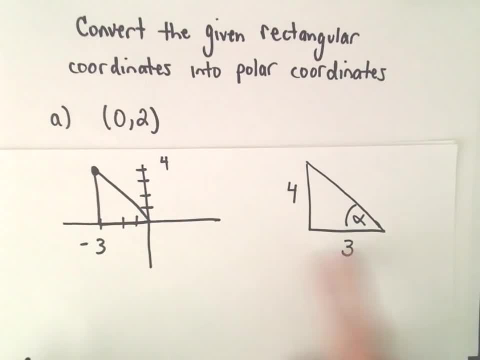 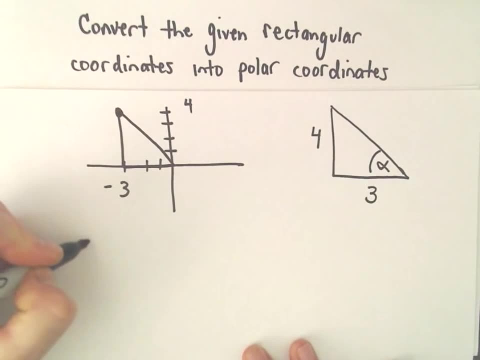 But on my triangle- I'm just going to label this, as you know- a length of 3. I can account for all the angles and all that in just a second. Okay, So to get the R value. so our R value would be the hypotenuse. 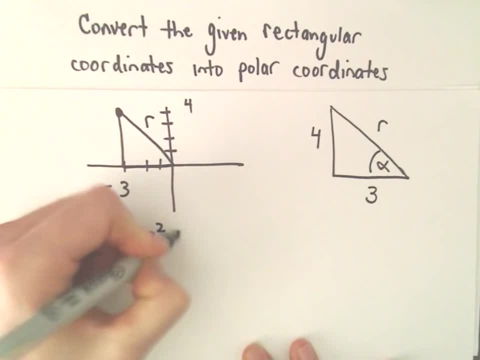 Well, R squared would be 3 squared plus 4 squared, just using our formula from a second ago. Well, that's 9 and 16, which is going to be 25.. Again, if we take the square root, technically you get positive and negative 5.. 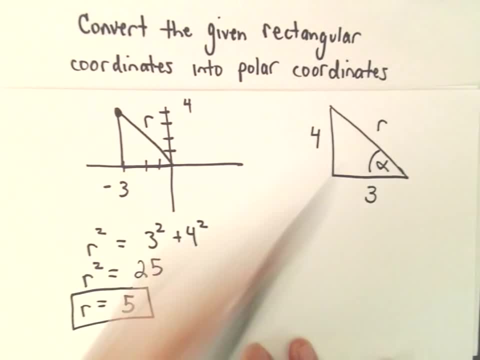 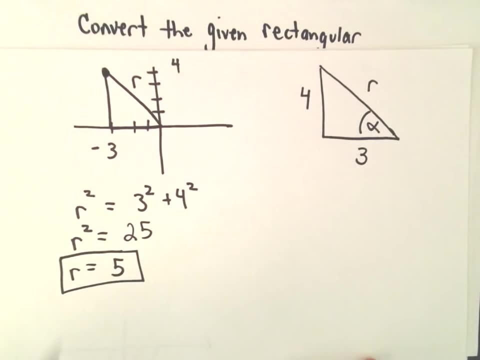 But I'm going to use the positive 5.. I'm going to make R equal to positive 5 in this case, And what I'm going to do next is figure out my angle alpha. Okay, So I'm going to figure out my angle alpha. 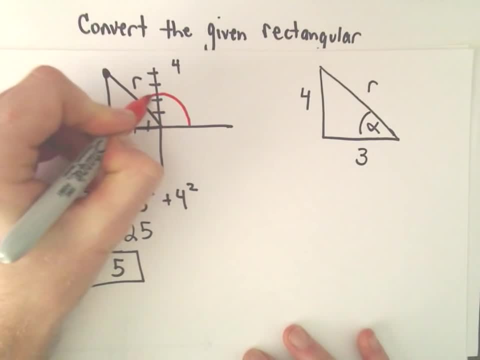 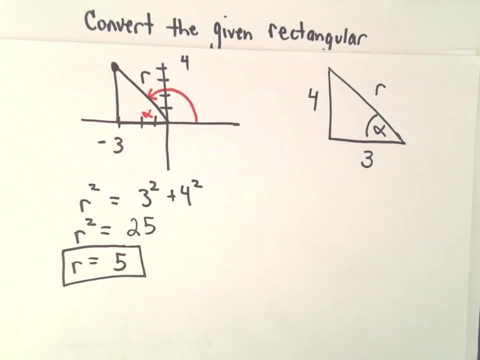 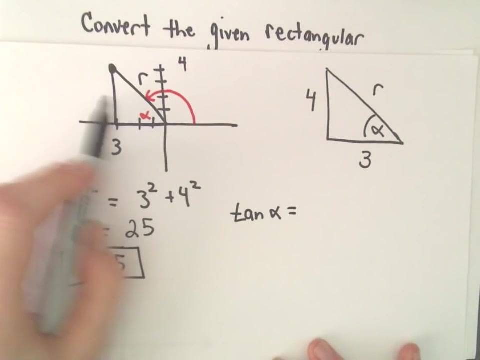 And then I'll take 180 and subtract that angle to get the angle that we're going to use when we use our polar coordinates. Okay, Well, tangent of the angle alpha. that would just be. so let's see what's tangent opposite over adjacent.